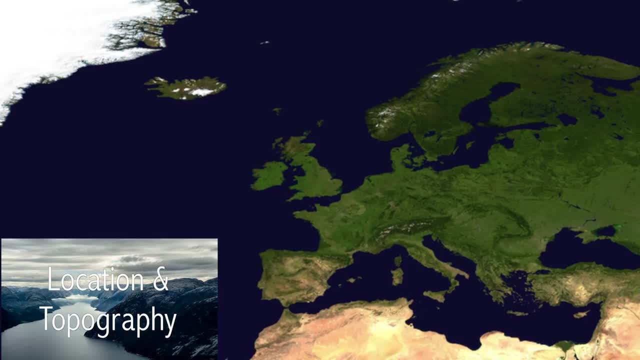 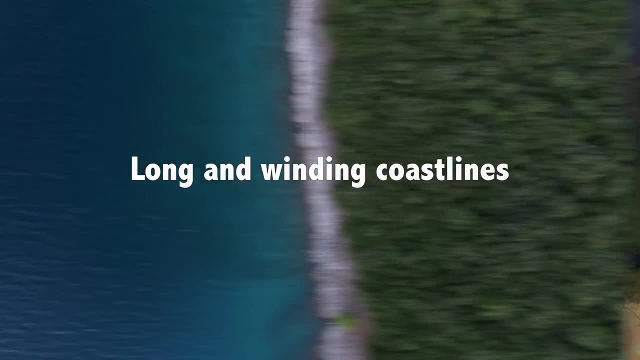 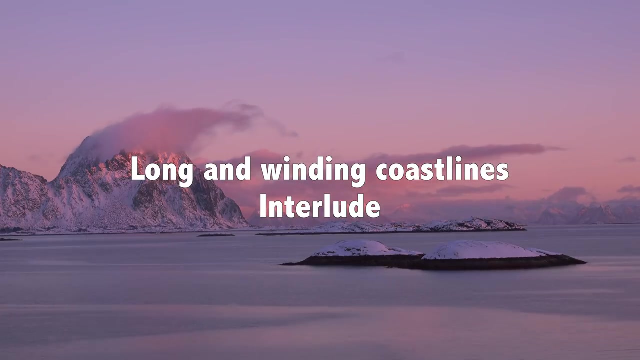 Reason number three: location and topography. Even though we're talking about a relatively small continent, Europe has broad access to sea, with long and winding coastlines in the south, west and north. These coastal areas are full of natural harbors, close to rivers which are long. 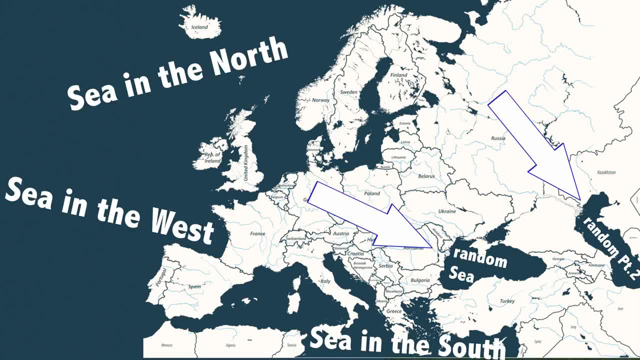 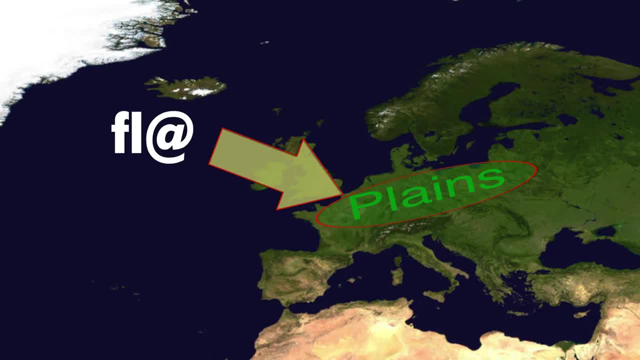 empty in different seas and connect with one another. All of this is great for commerce and trade. Furthermore, Europe's topography is also blessed with large flat plains, mostly in the north, again connected by rivers, and a convenient desert-like-thereof situation. 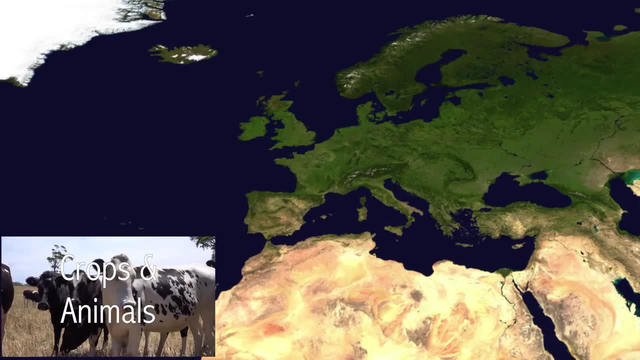 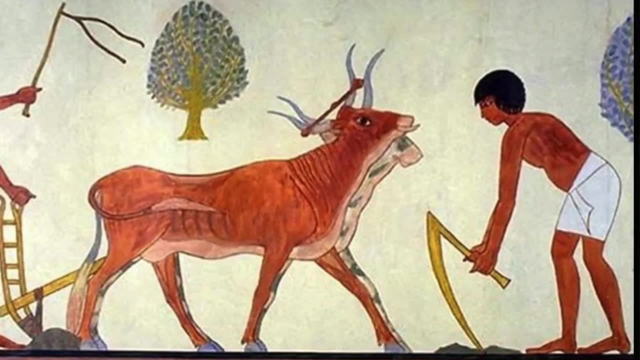 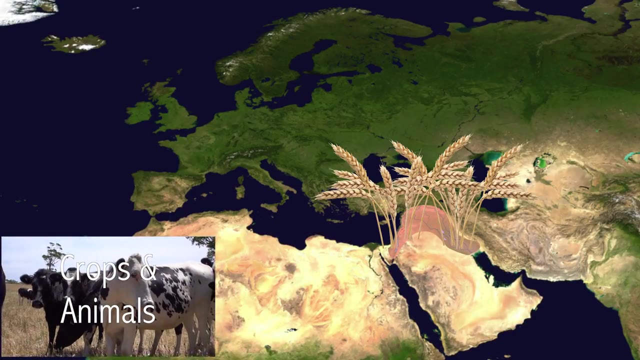 Reason number four: right: domesticable crops and animals. Thanks to its proximity to the Fertile Crescent, the birthplace of agriculture, Europe took advantage of the domesticable animals and crops that happened to be found in this area. In fact, all of the major five domesticable livestock now used worldwide—cow, sheep, goat. 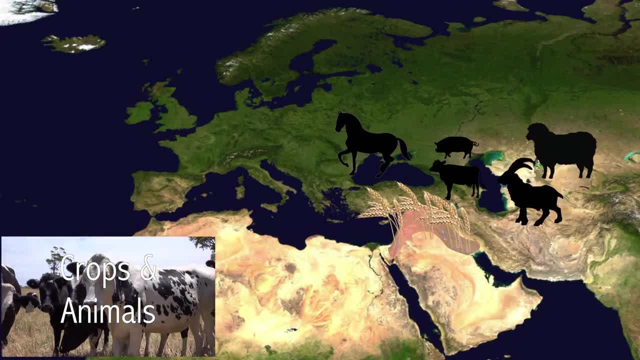 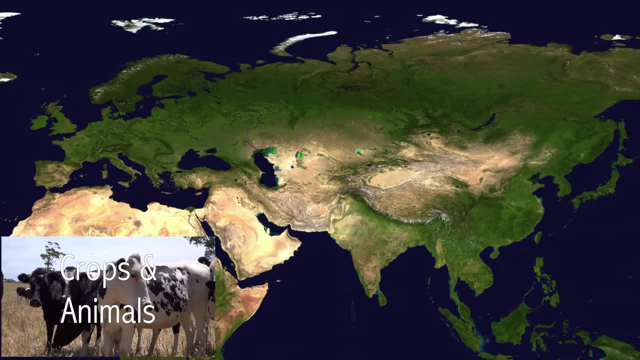 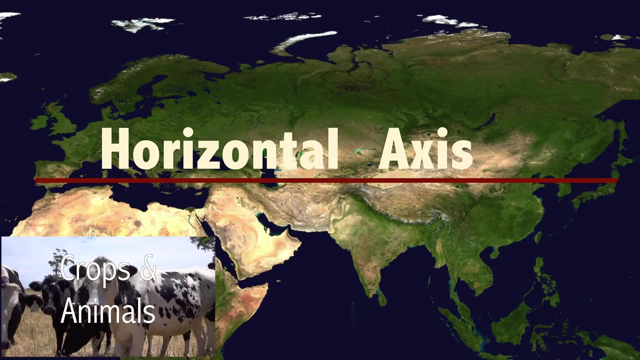 pig and horse—were found between southwestern Asia and eastern Europe because of luck. Furthermore, as brilliantly outlined by Jared Diamond in Guns, Germs and Steel, the Eurasian continent has a general horizontal. horizontal orientation, or, as called in the book, axis, which means that faraway locations have 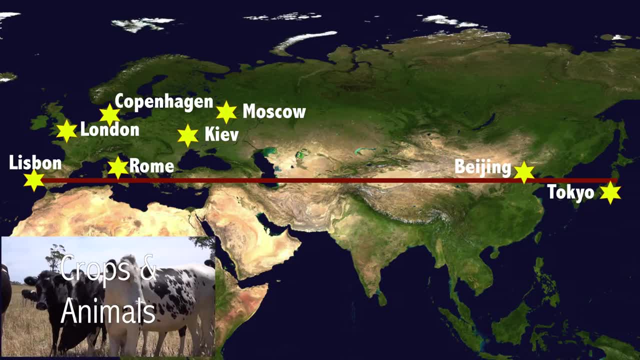 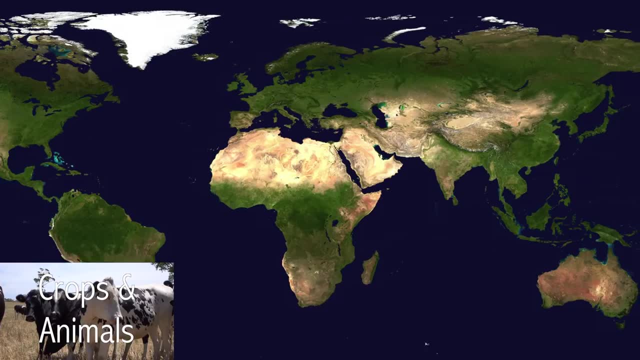 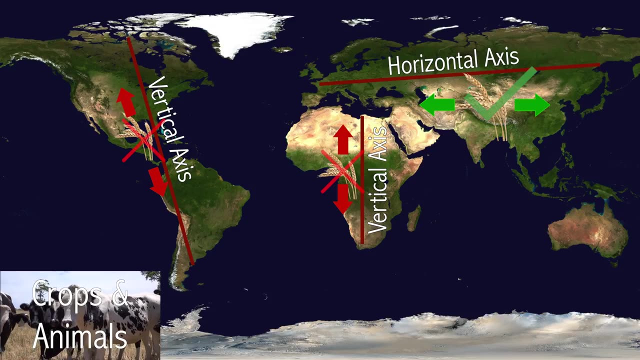 similar latitudes, hence similar climates and conditions, which allowed to grow and spread these domesticable crops and animals in different parts of the continent. Other continents could not do this because domesticable animals lacked thereof and general vertical axis made the spreading of crops near impossible. 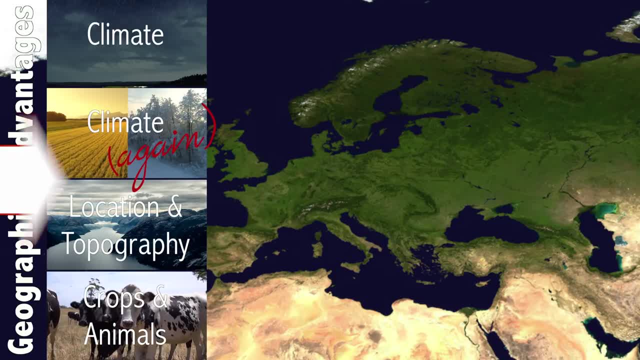 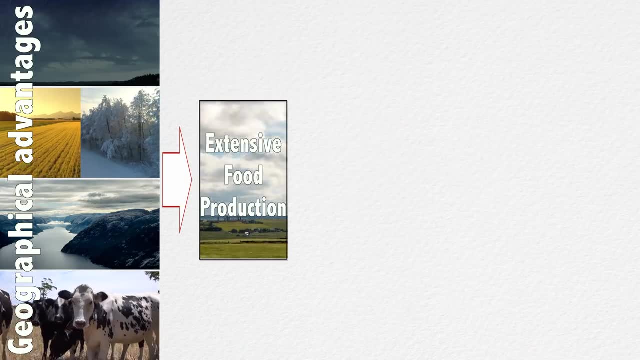 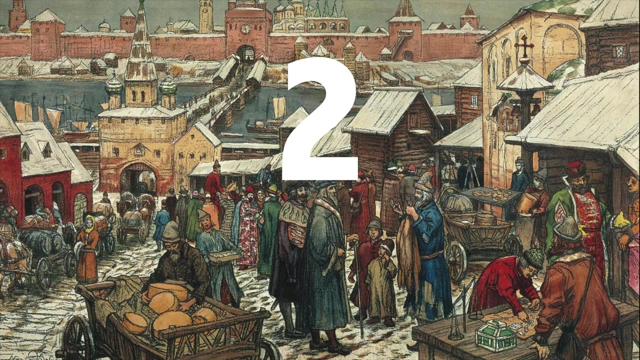 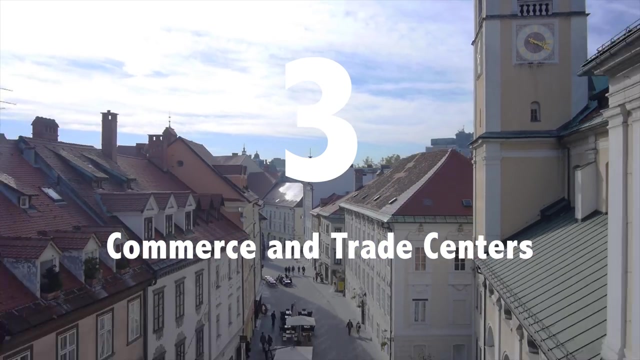 When combined, these precious natural features allowed for extensive food production in Europe, which resulted in: 1. Not all humans needing to work in agriculture, also known as human specialization and craft development. 2. Population growth and high population density. And 3. Its location and topography granted the development of commerce. 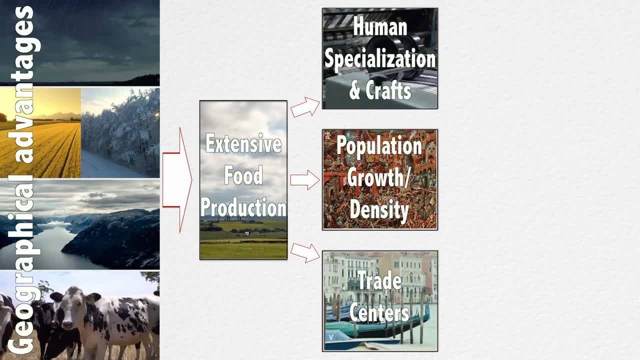 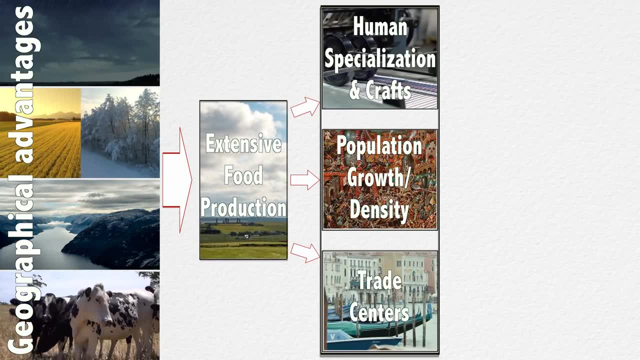 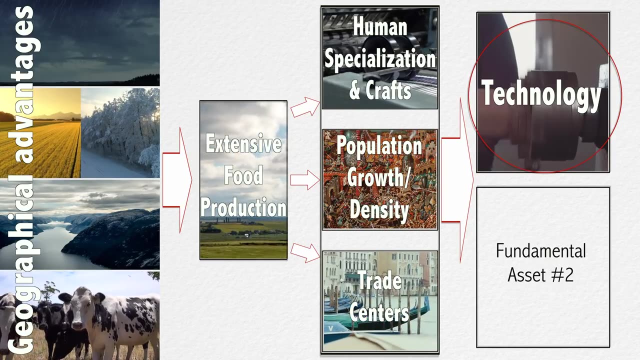 cities and trade centers, which are essential in order to redistribute the excess food production. Ultimately, these advantages contributed to two fundamental assets that developed in Europe before other parts of the world: Technology, which, over time, gets reinvested into even more food production. 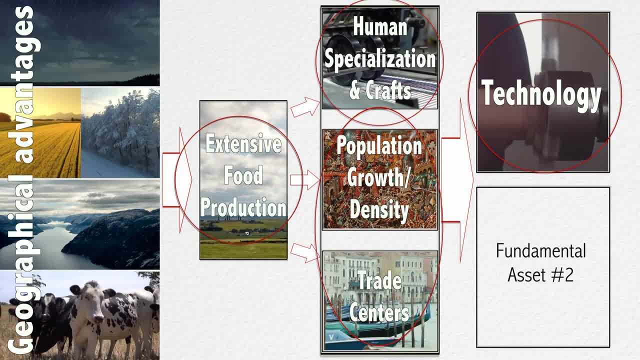 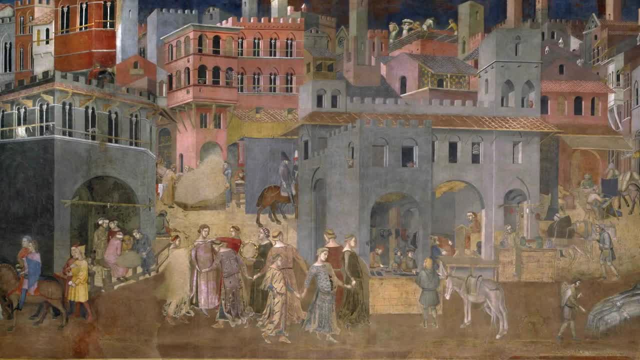 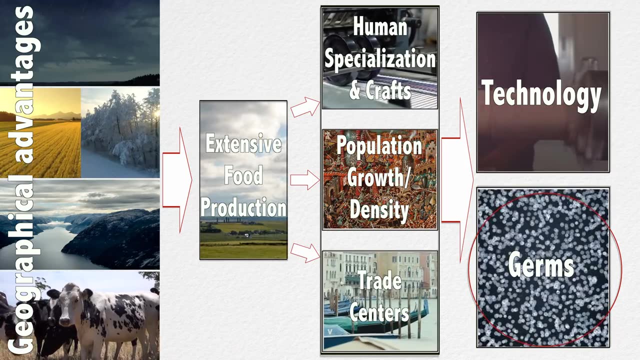 eventually rising standards of living of trade centers and speeding up human specialization and very important germs. This is the result of living in dense cities and trade centers with horrifying sewage systems and close contact with foreigners and livestock. This successful germ production will eventually wipe out. 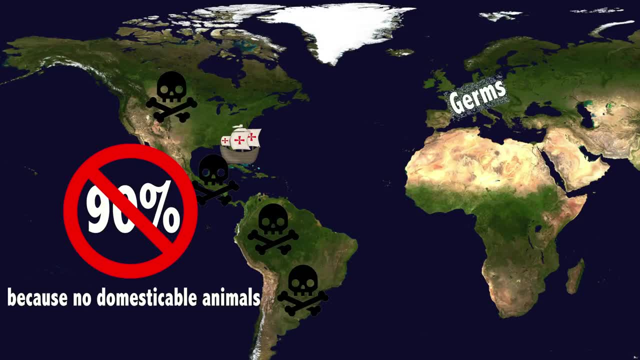 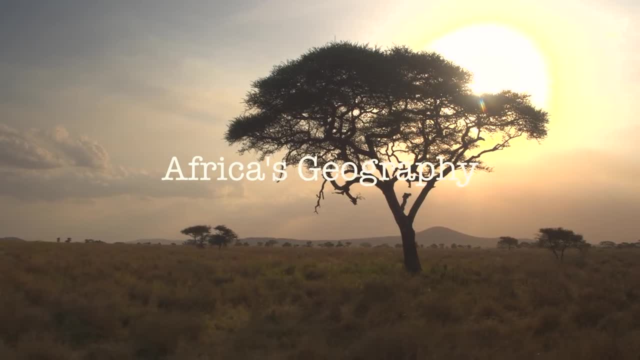 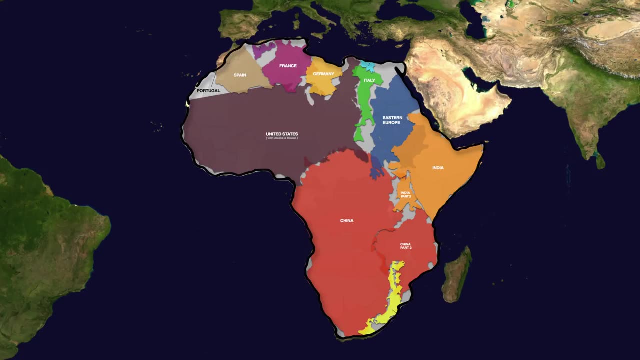 90% of the American continent's population. as if all of the violent murdering wasn't enough, Let's look at how Africa's geography compares. Unlike Europe, we cannot talk about one general type of climate in Africa, as Africa is huge And if we go back to that axis we talked about earlier, 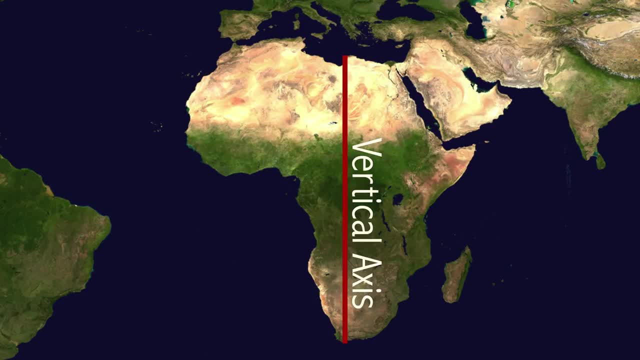 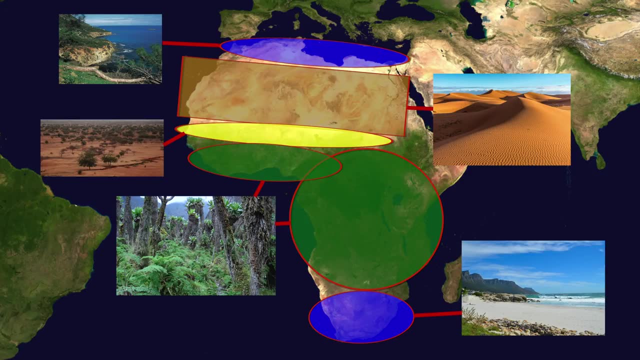 yes, being a vertically oriented landmass, we get the following climates: Mediterranean, desert, Sahel, deep forest. back to Mediterranean. This makes communication, trade and extensive food production near impossible. It has different climates, asks for different agricultural techniques and crops. 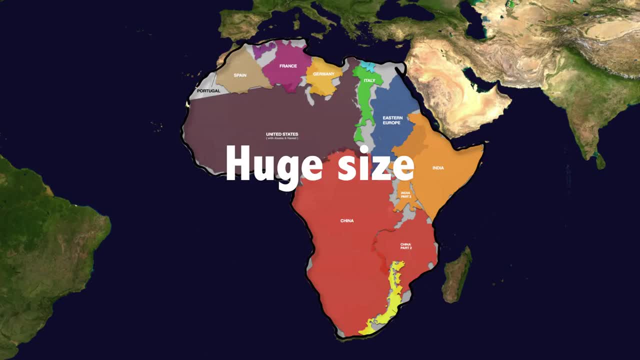 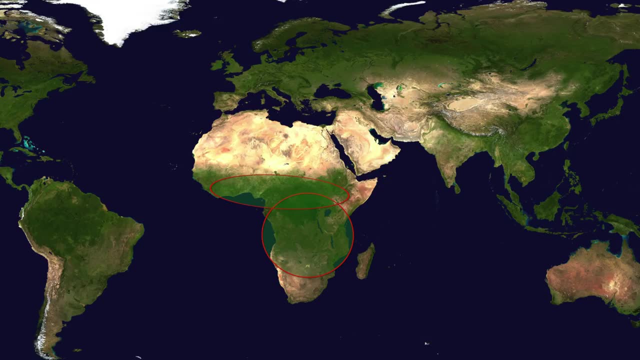 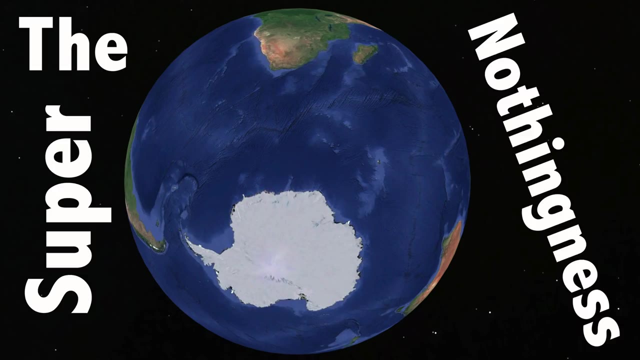 Africa has the strong problem of huge size paired with isolation. In fact, northern Africa aside, Sub-Saharan Africa developed in isolation to Eurasia Because of desertic nothingness in the north, Atlantic and Indian nothingness on the side and super-duper nothingness in the south. 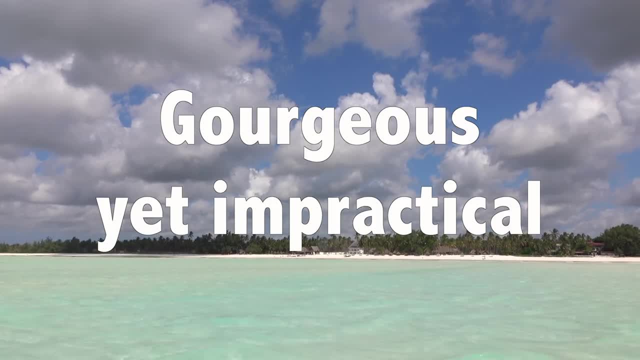 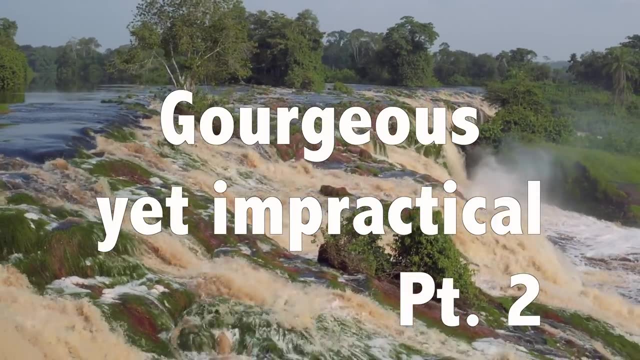 On top of that, Africa has terrible natural harbors, with coasts generally generally not being deep enough to dock ships, and rivers that aren't navigable due to gorgeous but impractical constant waterfalls. And finally, to make this even harder, in the 19th century, monkey-derived brains with slightly more advanced technologies due to fortune geographical advantages, decided to conquer the region and drew lines on Africa with little idea of what the continent was like in terms of cultures, ethnicities, geographies, et cetera. 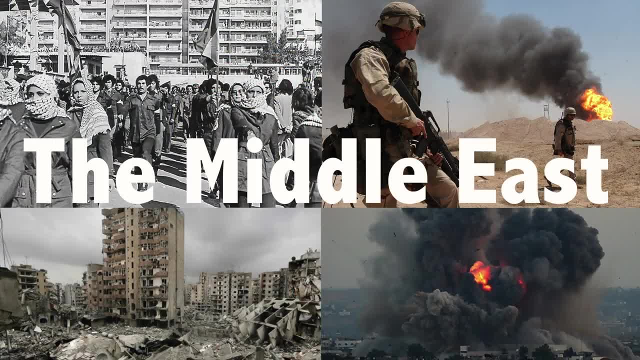 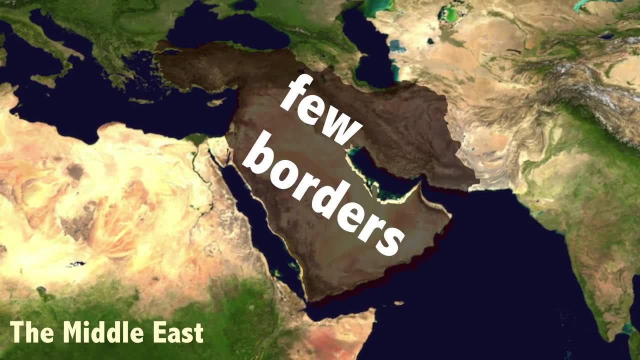 Wait, did someone talk about unfair colonialism? Well, let's discuss the Middle East. Just slightly over a century ago, few borders existed in this area. Space was governed according to geography, ethnicity and religion, without any sense of nation state. 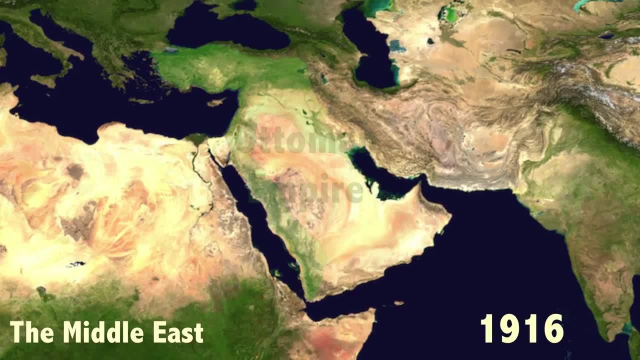 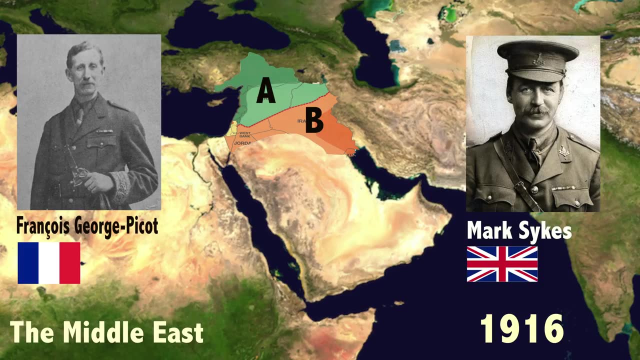 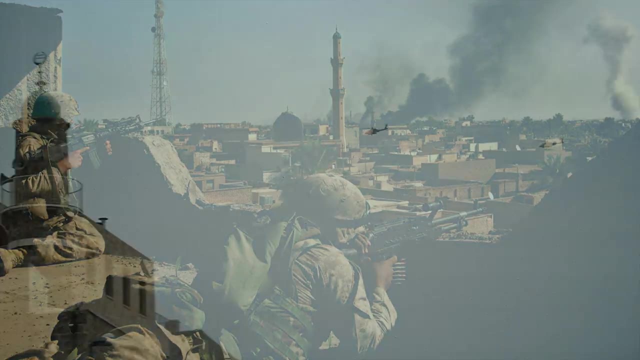 In 1916, when the Ottoman Empire began to collapse, the French and English had the brilliant idea of drawing the Sykes-Picot Line, creating the first ever artificial division in the region, which began a century of conflict and violence. Historians agree that the continent was extreme and violent. 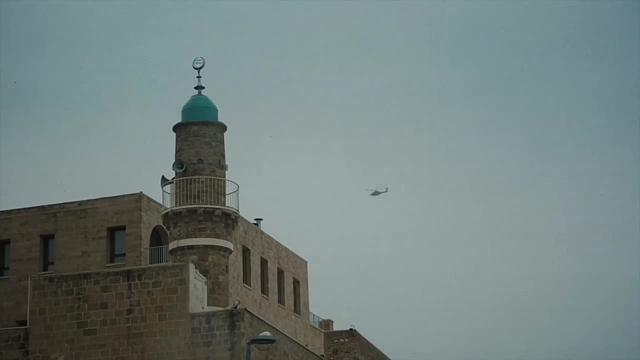 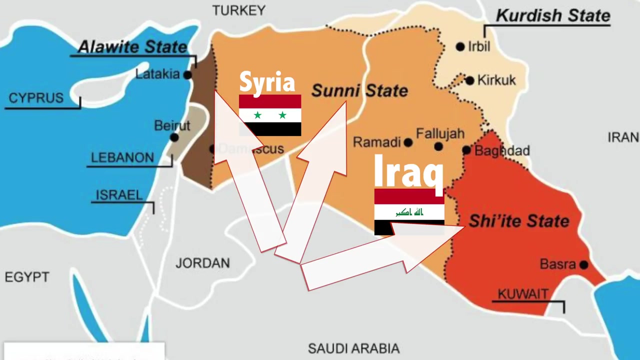 due to religious tensions before European interventionism. but drawing lines in the sand and putting people unused to living together from different branches of Islam under the same legal, political, economical system, invented by a different culture, is not a recipe for justice, equality and stability.